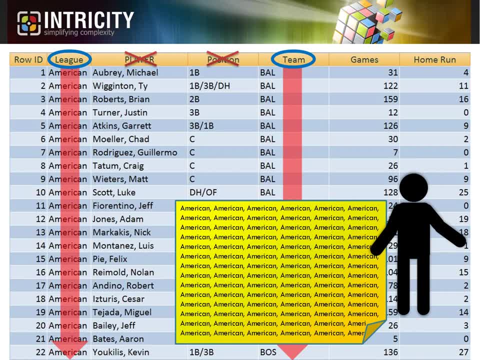 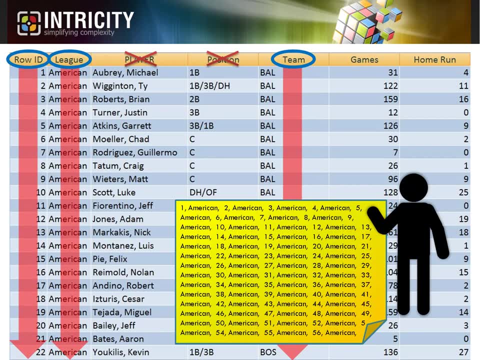 which league to assign each team it's retrieving. The way it does this is that the columnar database assigns a number to each row of data, allowing it to quickly pair up the many columns that it retrieves. You can see how this really comes in handy when you start reading the 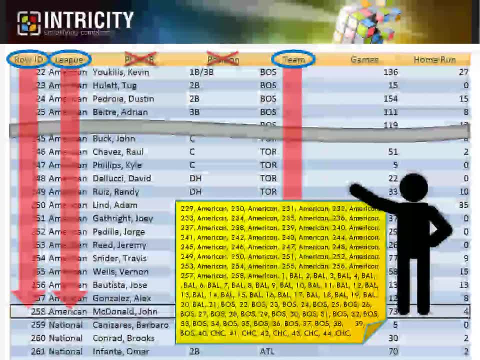 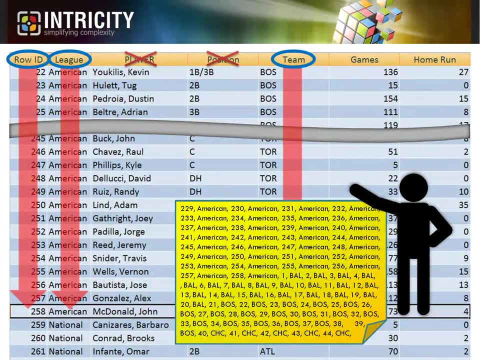 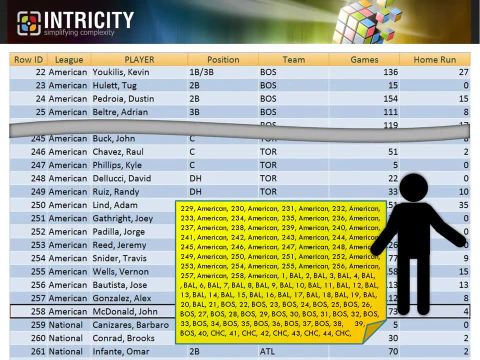 teams column. All it needs to know is which number the American League values ended at, In this case row 258, meaning I just need teams from 1 to 258.. Now you probably noticed how the columnar database was repeating American over and over. 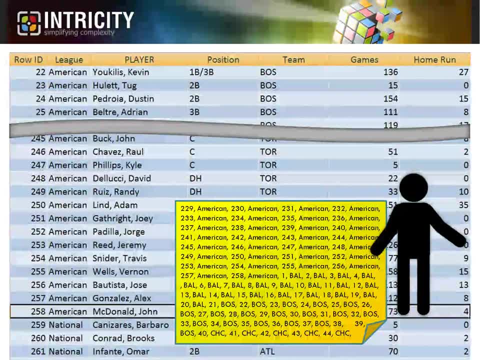 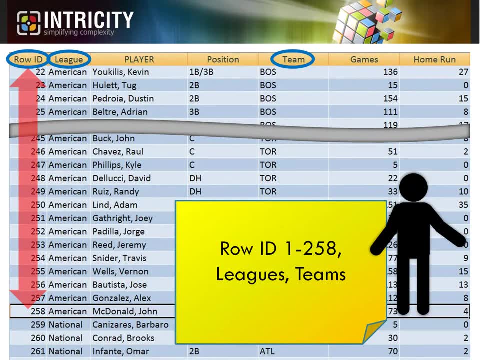 This is actually another advantage of the columnar database. By using the numbering system in the columnar database, algorithms can be used to simplify the retrieval of data, And you'll find that each columnar database system has highly sophisticated methods of gaining further performance measures. 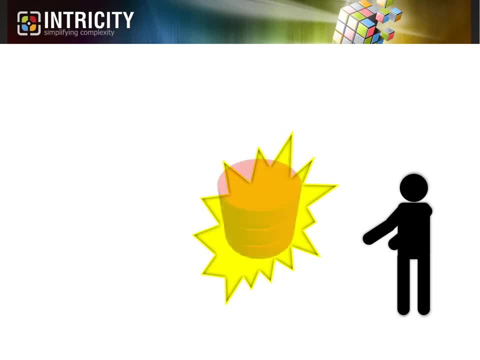 Knowing what I know now, I realized that the presentation I sat through a few years ago wasn't reading billions of rows of data. It was just reading a few long columns of data. Columnar databases can be a very straightforward way of addressing the mounds of data corporations. 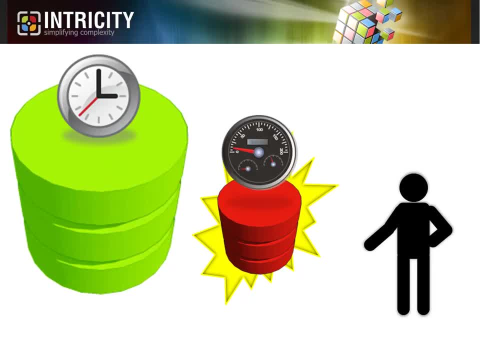 have to wade through. They're not a replacement for traditional databases, but certainly a powerful way of doing highly aggregated analysis. Intricity specializes in providing leading-edge solutions for today's complex data. If you're interested in learning more about the columnar, 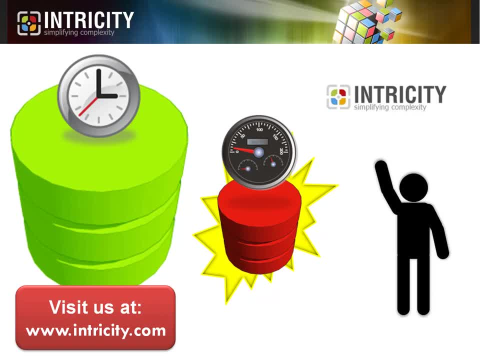 database: click the link in the description: data problems. I encourage you to visit Intricity's website and talk with one of our specialists, and I commit to you that we'll live up to our slogan of simplifying complexity.